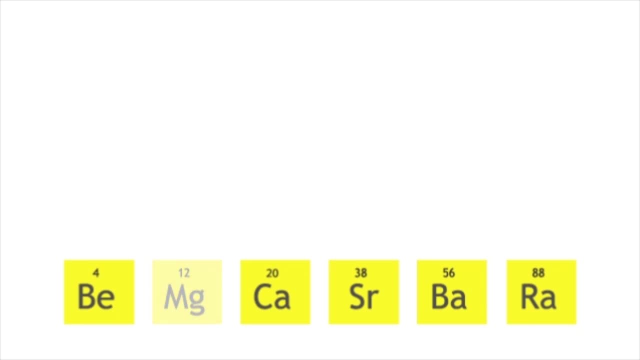 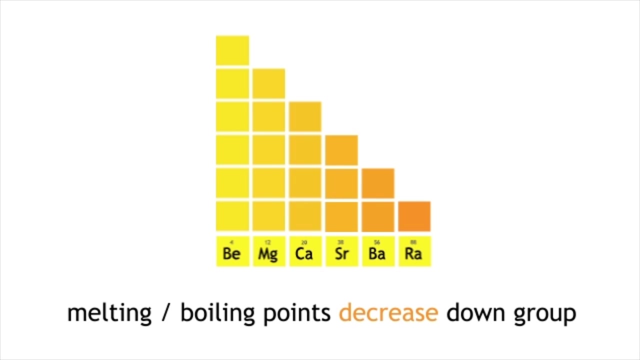 Like the alkaline metals, these metals, except for magnesium, are stored in oil. Similar properties and reactivity trends are also observed Moving down the group. their density and reactivity increases, Melting points and boiling points decrease and the metals become softer. 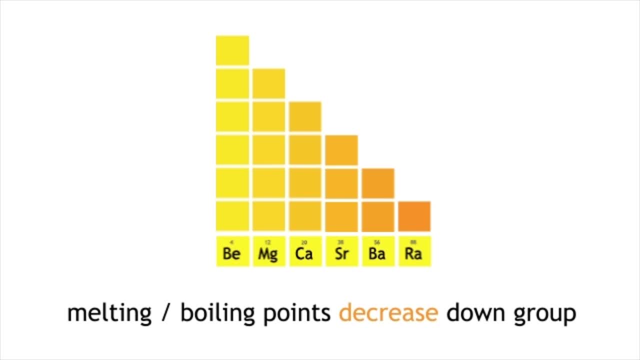 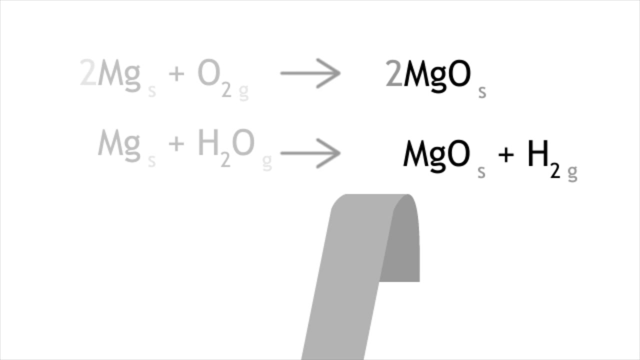 We will now learn about the reactions of magnesium and calcium with oxygen and water. Magnesium is shiny and silver, but you will see that your magnesium strip may be dull. This is due to the formation of an oxide layer from exposure to air. Simply clean it with steel wool so to remove as much of the oxide layer as possible. 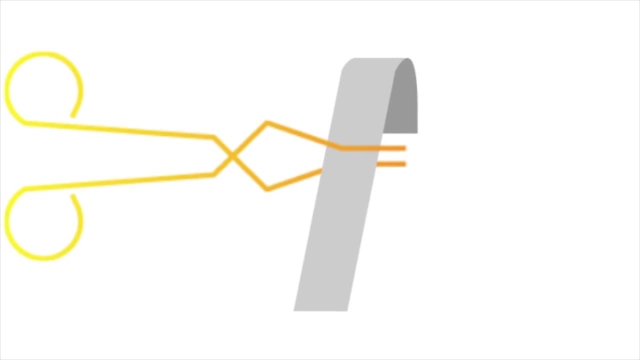 Using a pair of tongs, take the magnesium strip and hold it to a roaring Bunsen burner flame. The combustion of magnesium proceeds with a bright white flash. Take care not to look at this flash. This is the first time we have seen this. 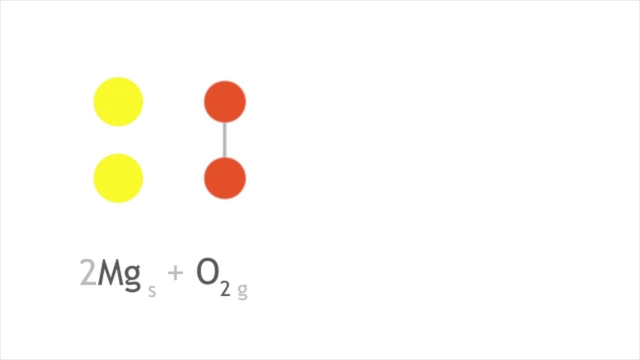 Magnesium reacts with oxygen to produce magnesium oxide, which is a white solid. Here is a challenge. Do you expect calcium to be softer or harder than magnesium? Please pause the lesson to think about this and resume when you are ready. Calcium is softer than magnesium. 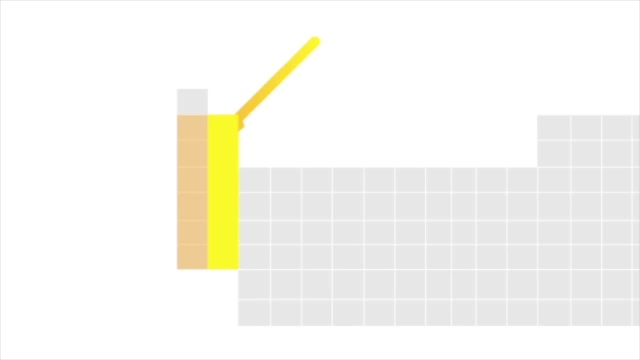 Moving down the group, the metals become softer. Overall, though, these metals are harder than the alkali metals. Calcium is also shiny and silver. Using a pair of tweezers, take out a chunk and cut a small piece using a scalpel. 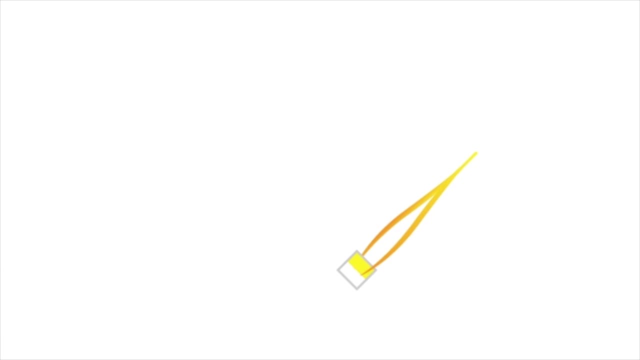 Remove excess oil using paper towels, Using tongs. place in a roaring Bunsen burner flame. You will observe that it burns with a red flame. Calcium reacts with oxygen to produce calcium oxide, which is a white solid. So magnesium and calcium react with oxygen to form their respective oxides. 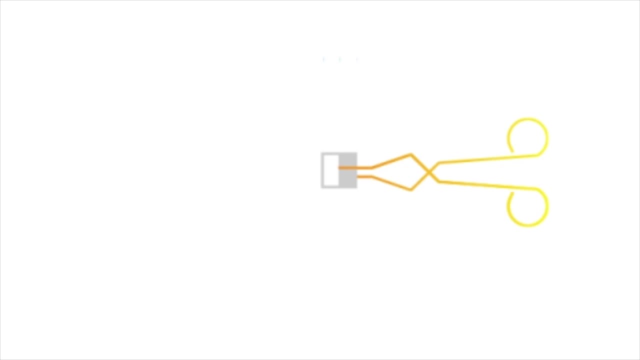 Let the formed calcium oxide cool. It is important that you allow it to cool sufficiently, because the next step is exothermic. Place the cooled calcium oxide in cold water. Calcium oxide reacts with water to produce calcium oxide. This is the first step.